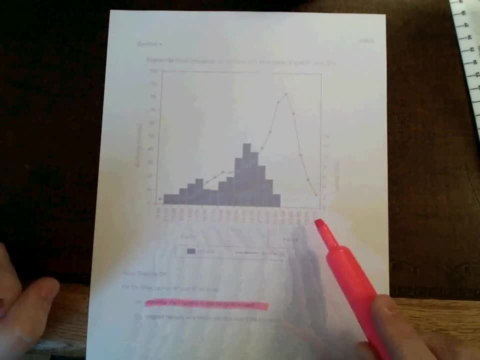 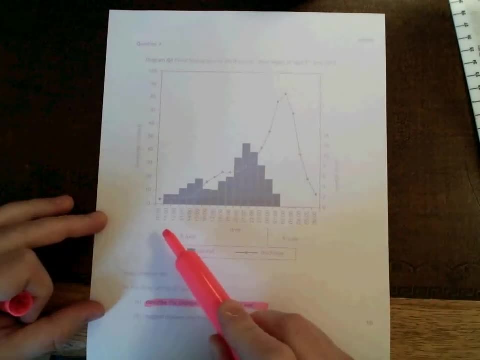 that has fallen over a period of time. Time is represented along the bottom of the graph. In this instance, this is the amount of rainfall that has fallen between 11 o'clock in the morning and 2am the next morning. You can see that the rainfall has got heavier and then lighter. 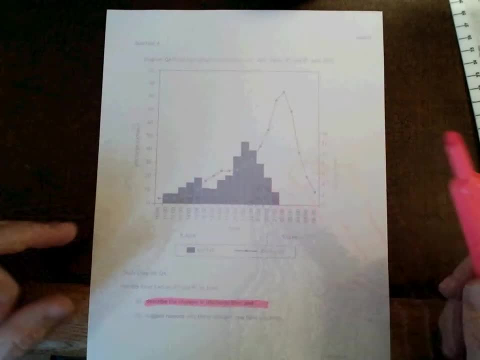 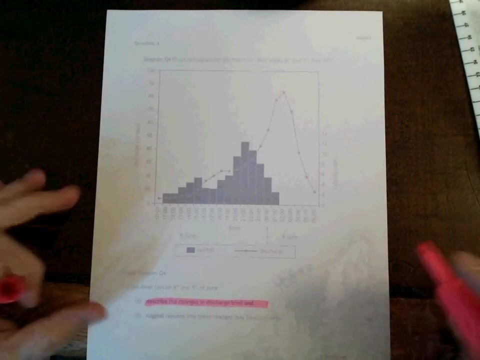 and then heavier again. So it would be reasonable to expect that this pattern of rainfall would have some impact upon a river in the drainage basin that the rain is falling over. It's your job to describe the discharge level. It's worth pointing out at this juncture that 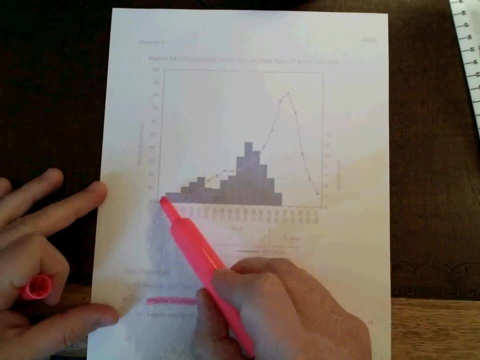 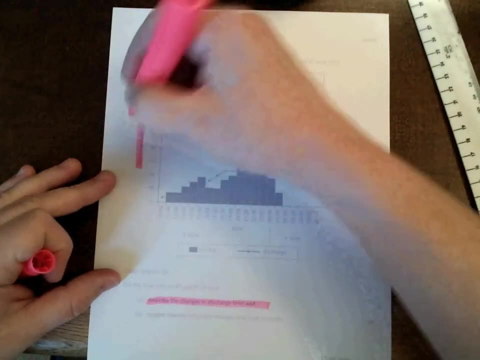 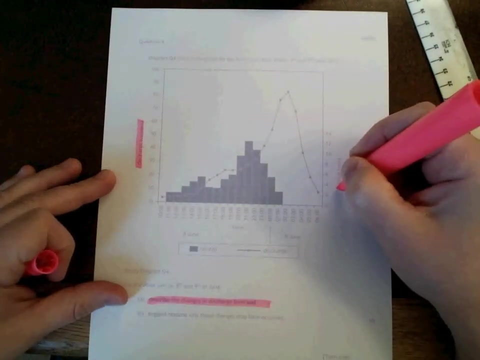 you're only going to score marks by describing the line on the graph. The line shows the amount of discharge and discharge is shown on the graph using its own key. Don't confuse the keys. The right hand side axis of the graph shows rainfall. We are going to use 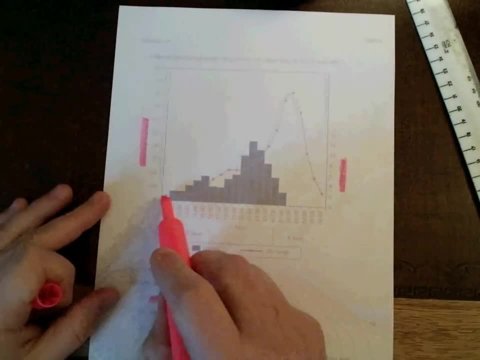 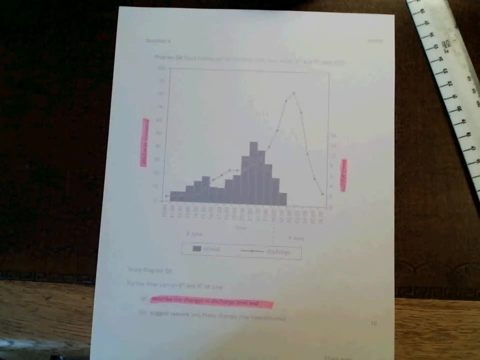 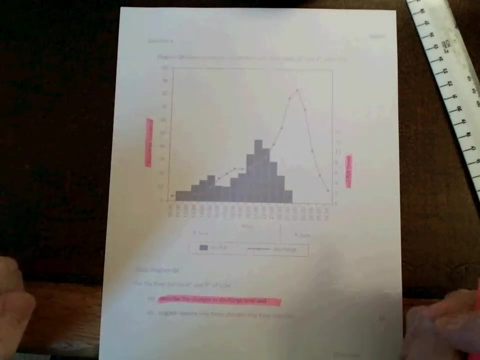 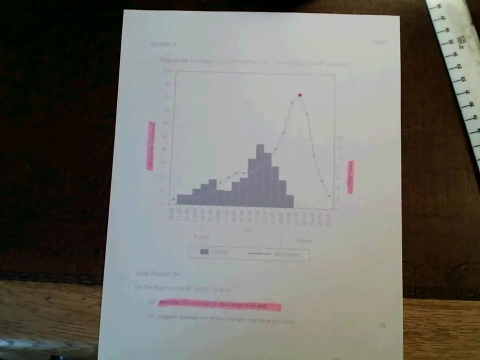 the discharge axis to describe the line that shows the rate at which the river is filling up with water. So let's look at that line. There are three basic elements to the line. I'll start with the easiest Here. At this point you can say the river has reached its peak discharge. 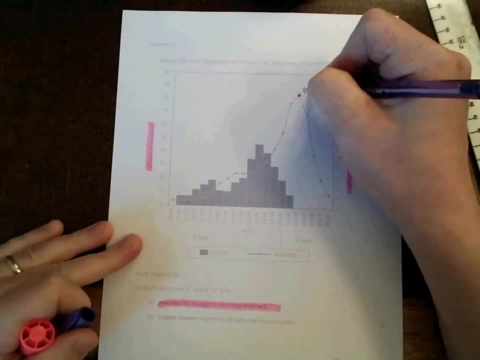 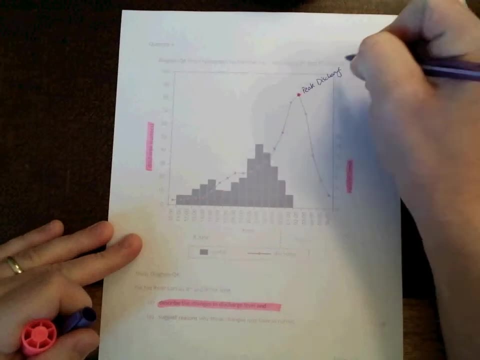 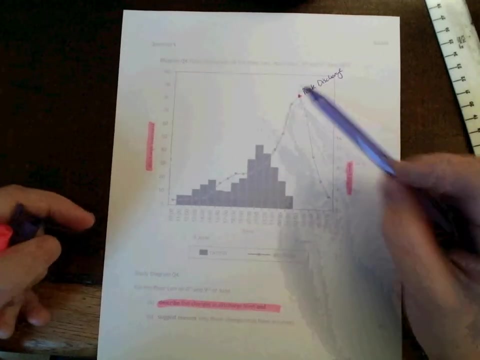 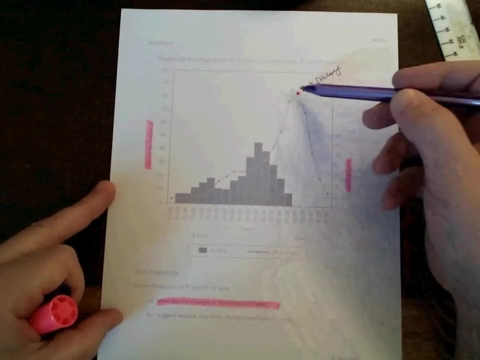 And if I were you sitting in an exam hall or doing an assessment, I would be annotating the question paper in exactly this way. The peak discharge is where the river reaches its highest point. If you can work out what time that took place and, just to really secure the marks, how much the discharge was at that. 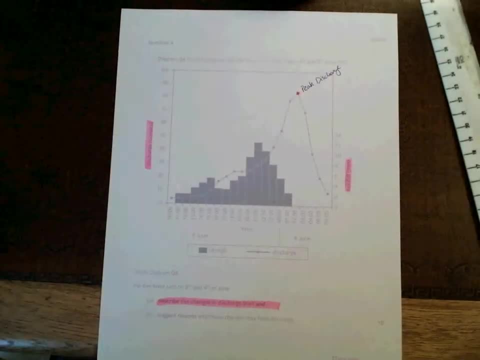 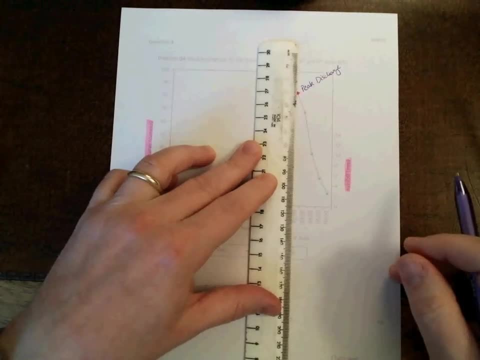 clean and do write writing. So basically students can do finite referents. one is for being able to write the math, one is for έχει. In the exam you need to write the exact answer to make the words that are vague in. 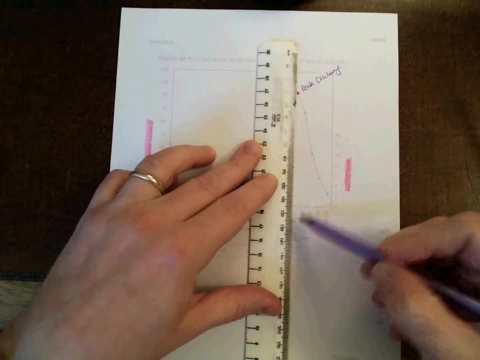 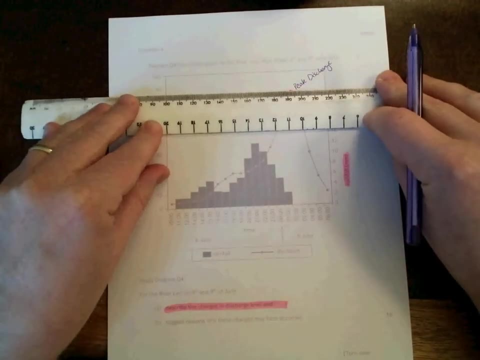 a very kind order. Again, you could see the right answer: why the B expected, why the practice and why the results are delayed, why the answer is lower or why the answer is drop at about 2 am. So what will you use for your distance learning? 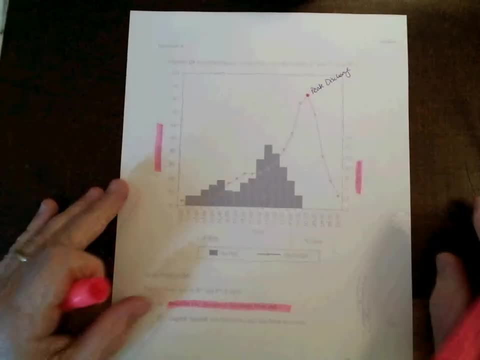 So what you do is you copyok, you convert the answer to a problem, for example a problem to be solved. So I'll now go ahead and type it. And that's because the falling limb tends to be after the peak discharge. 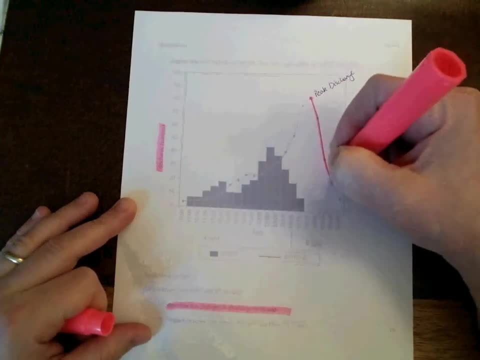 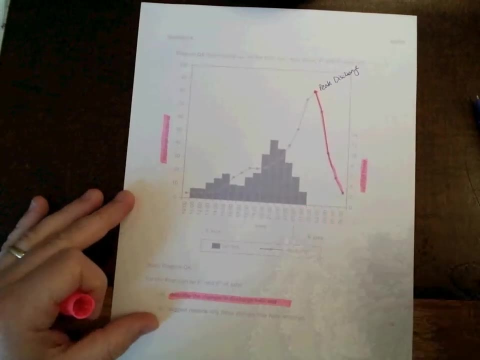 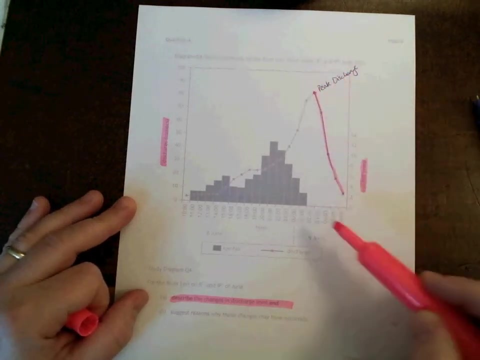 So that is this part of the graph. Now the falling limb happens between 2 am and 6 am in the morning And better still, I could add that it falls from 85 cumex approximately to 10 cumex approximately. 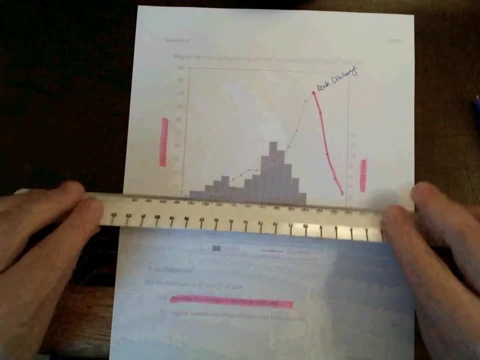 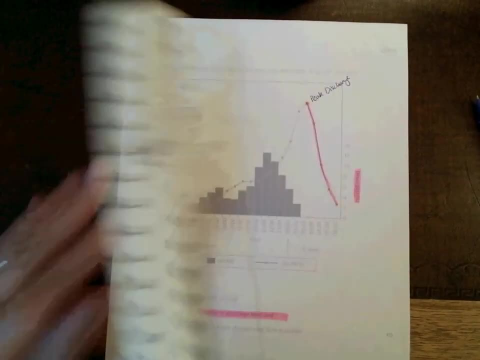 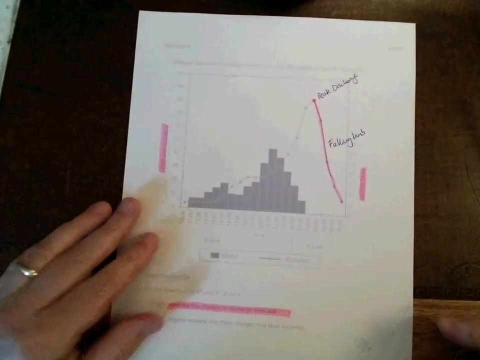 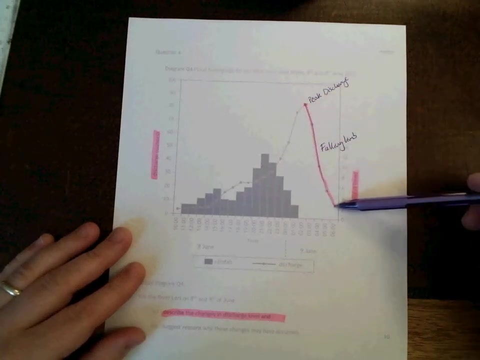 And I can check that I'm right about those values just by quickly lining them up with my ruler. So the falling limb is quite easy to spot. It represents the speed at which the river is returning from a peak level of flow to its normal level of flow. 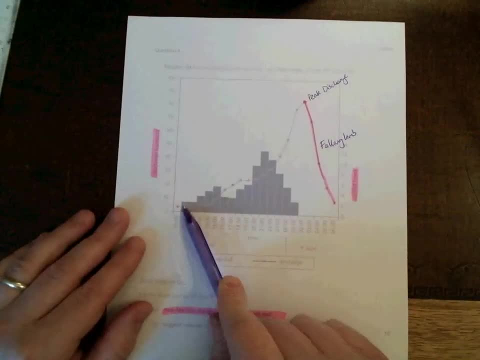 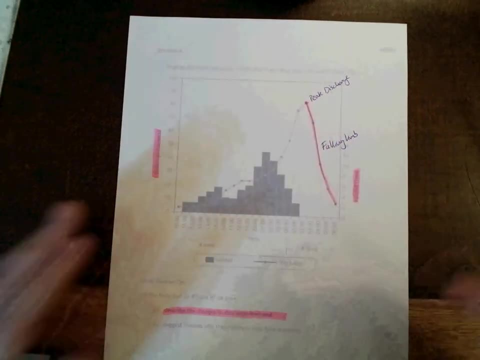 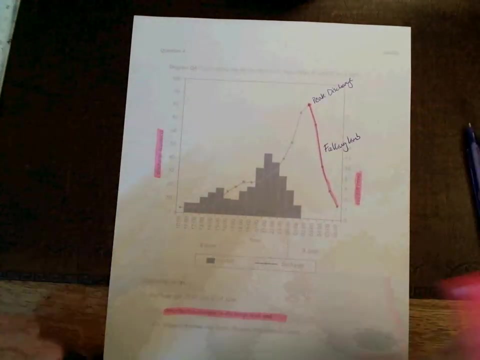 The rising limb is a term we use to describe the approach towards peak discharge, But it would be a mistake just to think of the rising limb as just one line that we can describe in a simple statement. In actual fact, this line has numerous things that we can point out. 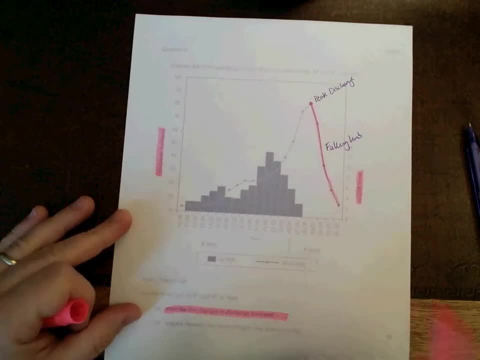 For example, there is an element here of your judgment involved. But at this point on the graph between 11 o'clock and 2,, there is a very graphic gradual increase in discharge. I will score a mark for pointing that out. 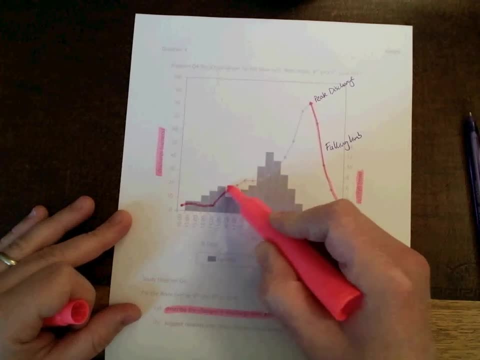 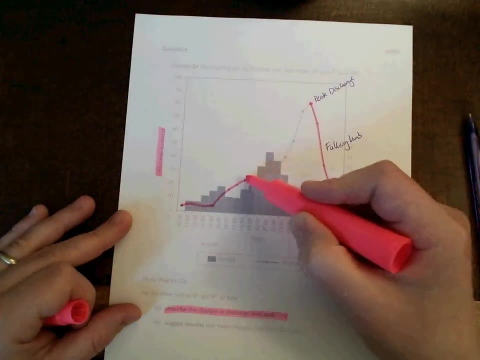 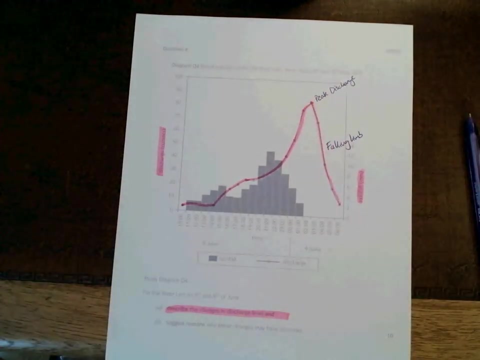 Discharge increases in speed between 2 o'clock and 6 o'clock And then rapidly increases between 6 o'clock before reaching its peak at 2 am. So you can see that actually I've made three observations on the rising limb. 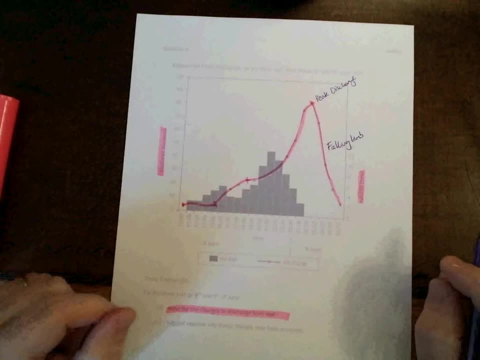 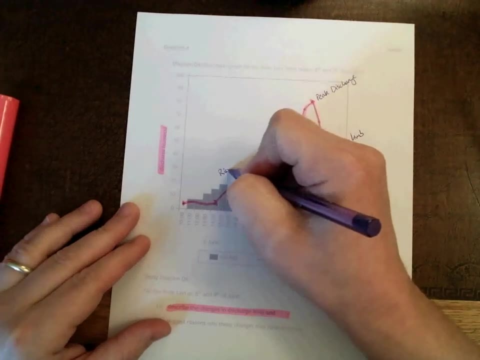 And you should be alert to these kind of fluctuations in the rising limb And you should make an effort to try and break it down and describe it in the way that I've just done. So the rising limb actually has the potential to score you multiple marks. 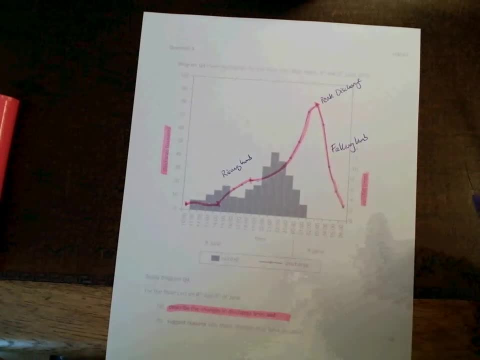 Okay, There is another element that we can, we can describe, And that's the lag time. Now, some people find lag times to be a bit confusing, But there's a simple method you can use to simplify them. Find your peak discharge. 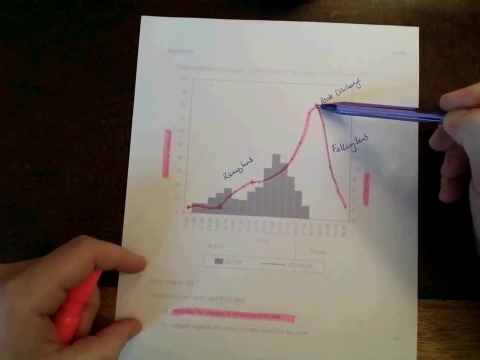 This is the point of peak discharge. here I've already described that. It's the point at which the river is fullest. Now, what we're really looking for here is the distance in time between the last heavy, the last peak in rainfall and this peak in discharge. 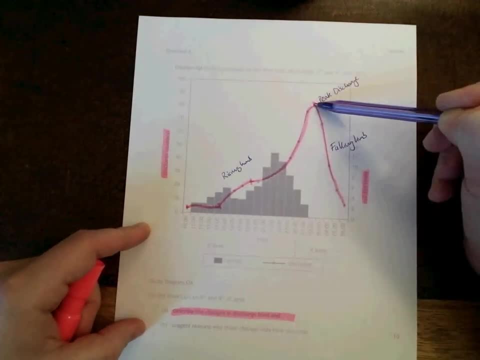 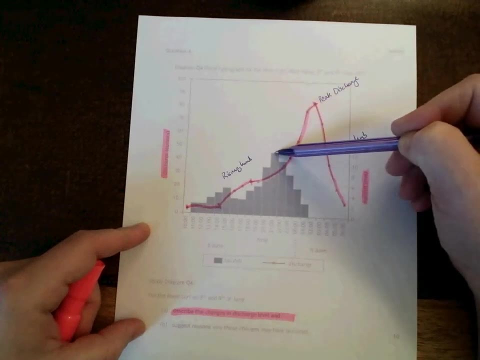 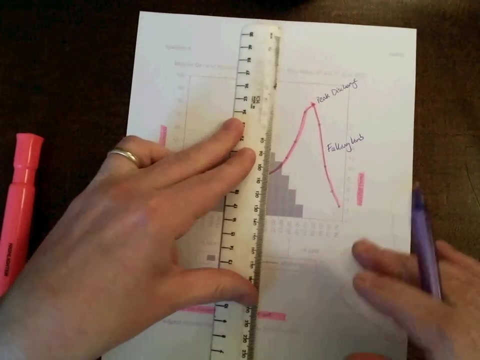 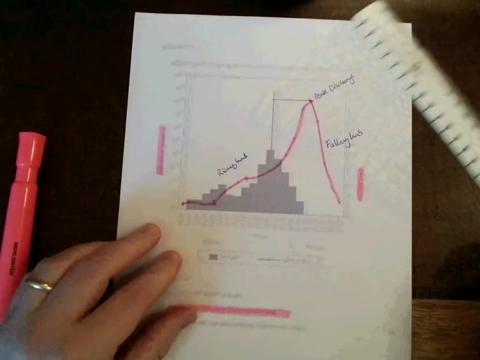 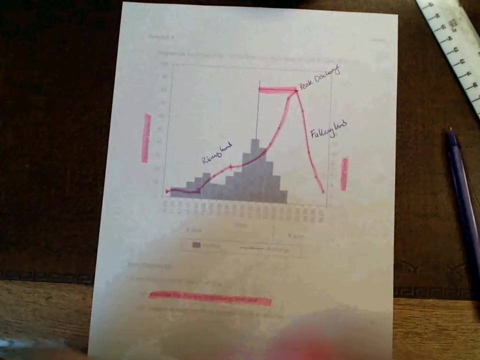 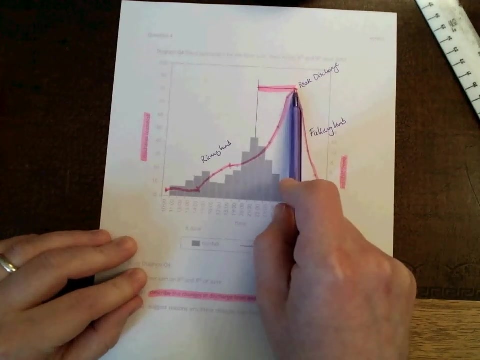 So you're going to work your way backwards across the graph from the peak discharge until you are over the most recent peak in rainfall, Which is this one. So, again, just by using your ruler, we're interested in this line here. This distance represents the distance in time between the river being at its maximum flow. 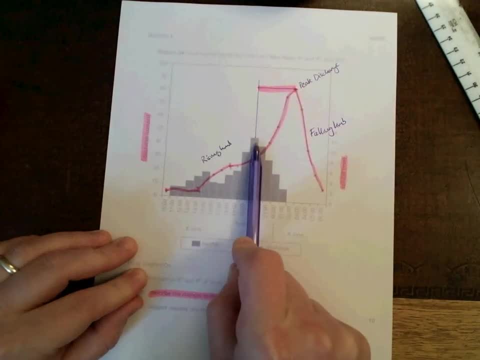 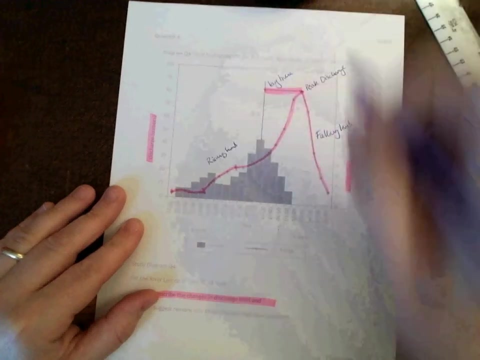 peak discharge and the rain being its heaviest, And that is, Let me just work this out- One, two, three, four, five. There is a five-hour lag time. This is a very important part in this problem, And it's the one that's going to help us find the right answer. 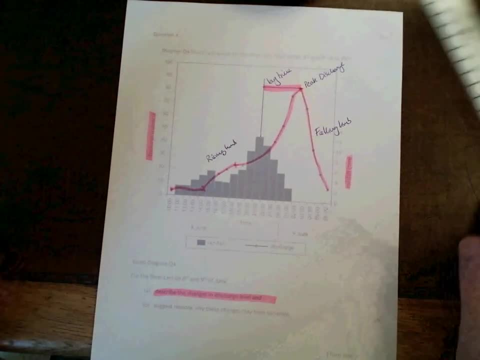 By taking this approach and breaking the graph down into parts using a highlighter and a ruler, you'll make your life a lot easier. You can also score in this question. this question is worth ten marks, So that is five marks out of ten. 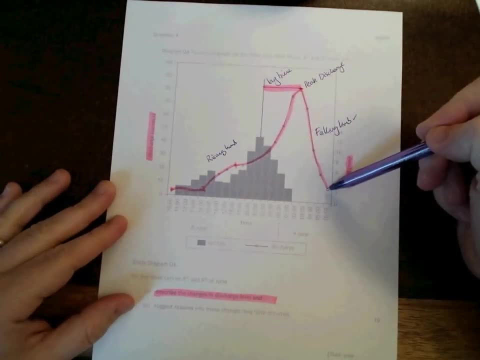 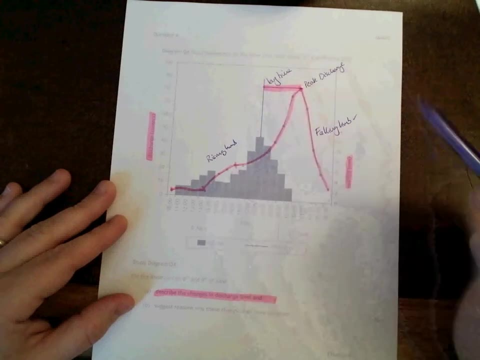 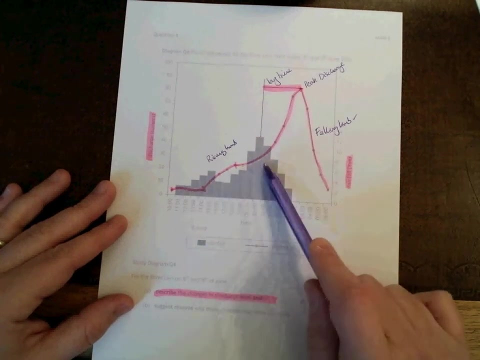 One for identifying when the falling limb begins and ends, One for identifying when the peak discharges, One for identifying the distance in time between the river and the peak length of the lag time, and one for any of the various valid descriptions in the. 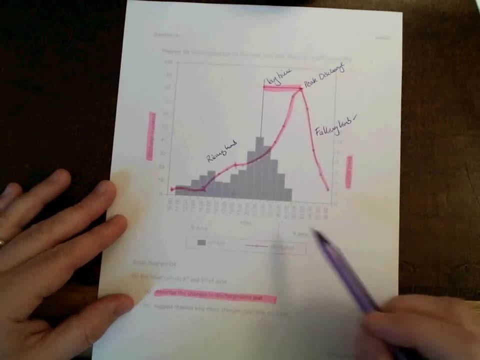 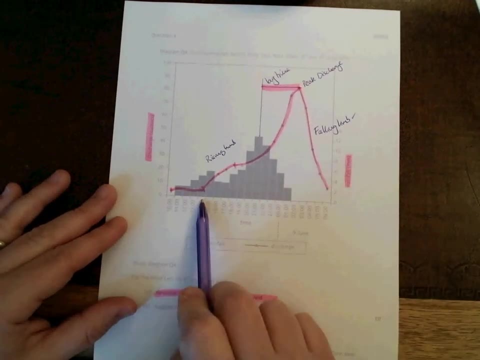 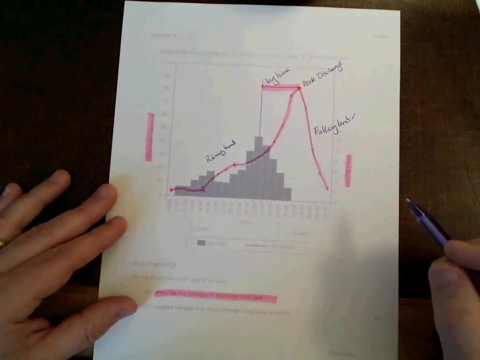 rising limb. try to be specific. use the values from the graph. if it were me setting this assessment, I would not only quote the times that these various events are taking place, but also the discharge quantities. and one final word: when describing the rising limb, notice my word choice, and this is why I said: